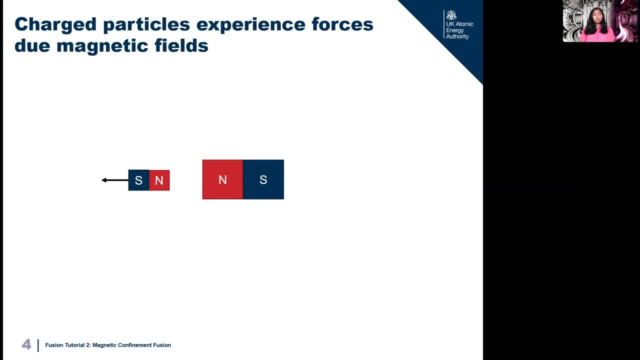 repel each other And therefore we can draw an arrow in this direction, showing that the smaller bar magnet will be repelled by the larger bar magnet. Now, if we place a bar magnet like this, we can have a guess at how it will behave. So the two North Poles. 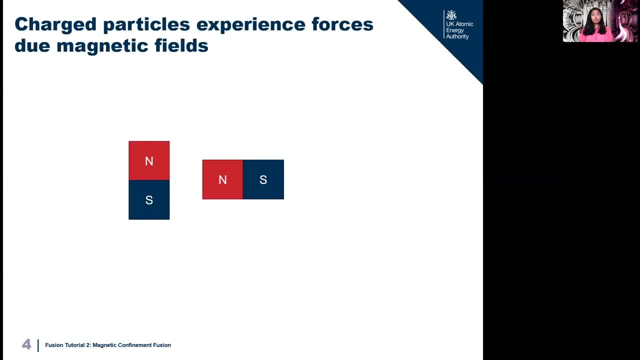 will repel each other, as like poles repel, and the two North and South Poles will attract each other, causing a rotating motion like this. We can use this rotating motion to our advantage by drawing an arrow in the direction that the North Pole ends up facing. 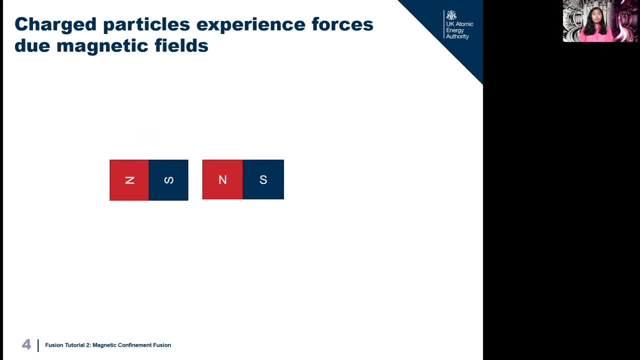 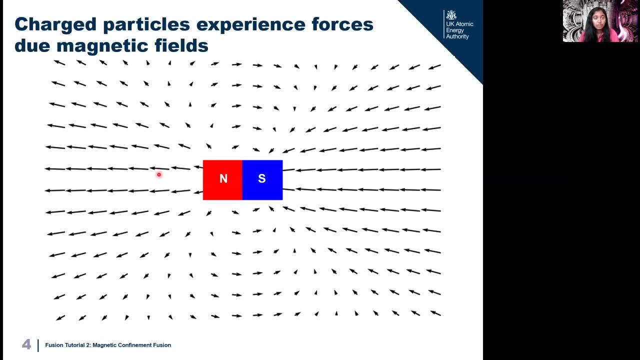 And this way we can draw arrows representing a magnetic field due to the bar magnet in the centre, And if we do that, it would look a bit like this. So, as we showed earlier, the North Pole faces away from this North Pole as opposite, as sorry, like poles repel. 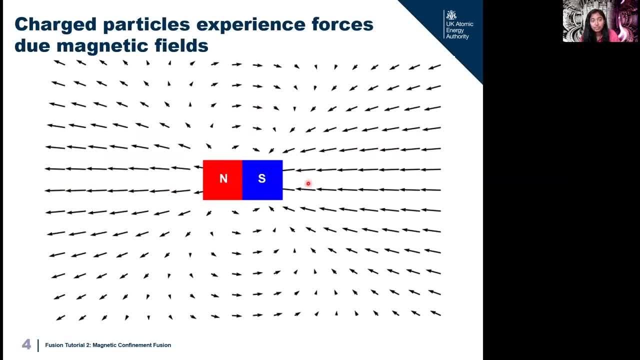 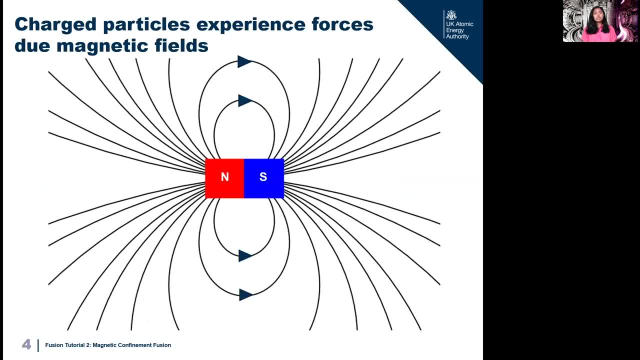 each other, And the North Pole, instead on this side, will be facing towards the South Pole, as opposites attract. If we join up all these little arrows, we'll get a diagram that looks like this, And this is how we draw magnetic fields in practice. 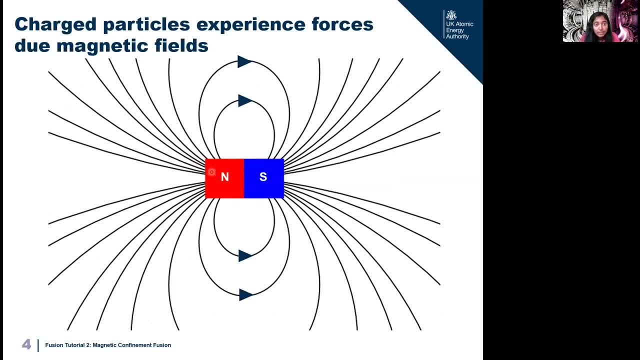 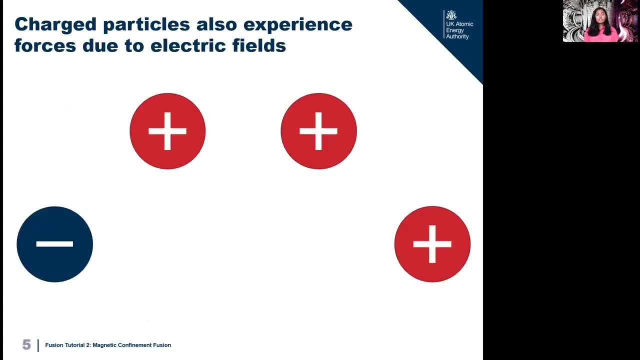 Note that the magnetic field lines loop from North to South, as you can see here, and down. here as well, We can treat charges in the same way that we treated the magnets, and charged particles also experienced forces due to electric fields. So if we use the same theory from: 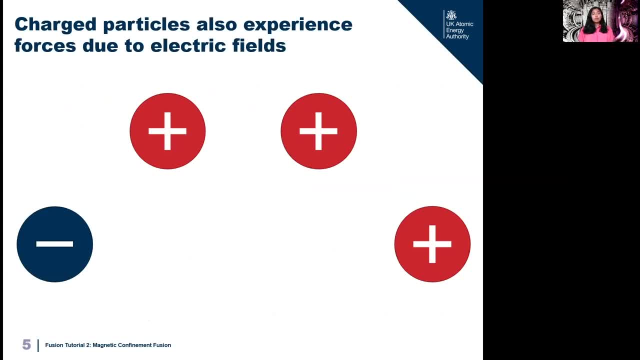 earlier of opposites attracting and, like things repelling. we can predict that the two charge particles at the top will repel each other. like so, because they have the same charge and the two oppositely charged particles will repel each other, So we can use the same theory. 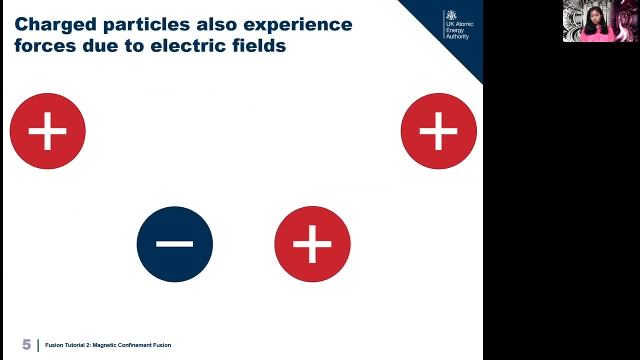 if I could. And this is how we get the same charge, but we can use the same formula. So thank you, Bye, bye. particles below will attract each other. We can use this theory again to draw electric field lines in a similar way to the magnetic field lines that we drew. 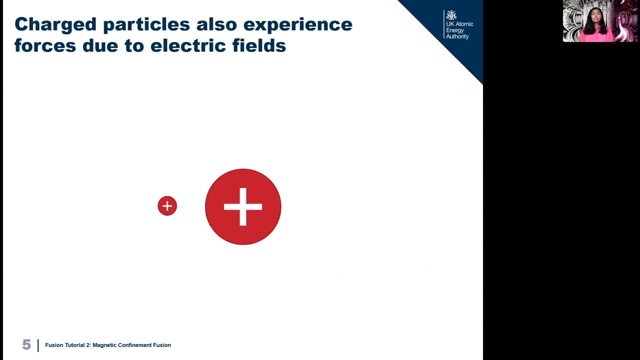 earlier, and we do this by placing a positively charged particle as a test charge particle in this environment and seeing how it behaves. Using the theory from before again of like charges repelling each other, you can draw an arrow in this direction, showing that the smaller test charge particle will be. 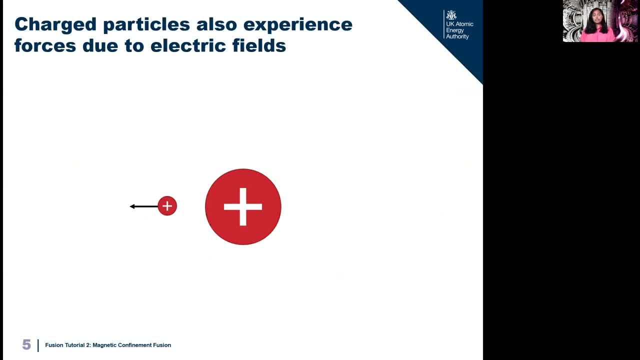 repelled away from the larger positively charged particle. We can place this test charge particle at multiple different positions around the positively charged particle in the center and see how it behaves and draw arrows in the direction that it moves. If we do this at every position around the 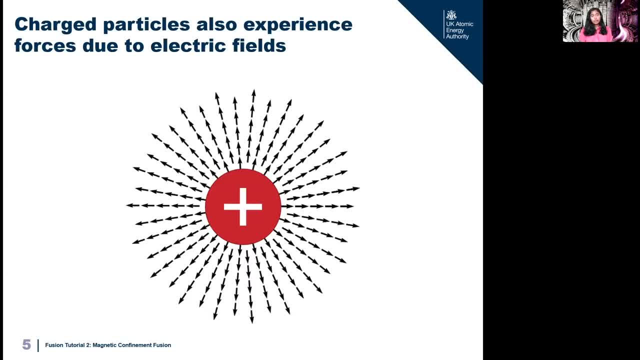 positively charged particle in the center, we'll get a diagram that looks like this. and if we join up the little arrows together, like we did before with the magnetic field lines, we'd get a diagram that looks like this, and this again is how we draw electric field lines. 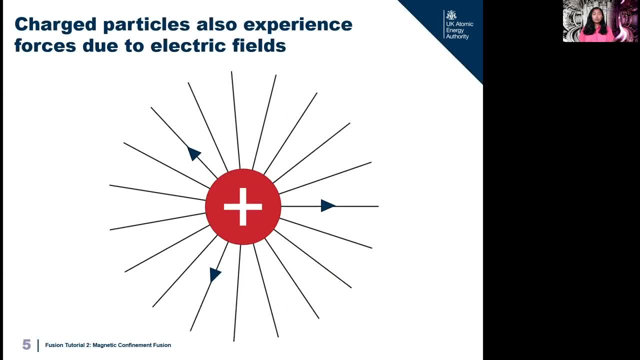 In practice. note that the arrows are all pointing outwards, and this is because we placed a positive test charge particle in this environment and this positively charged test particle will be repelled away from the positively charged particle in the center and therefore the arrows are pointing outwards. If, instead, we had a negatively charged particle in the 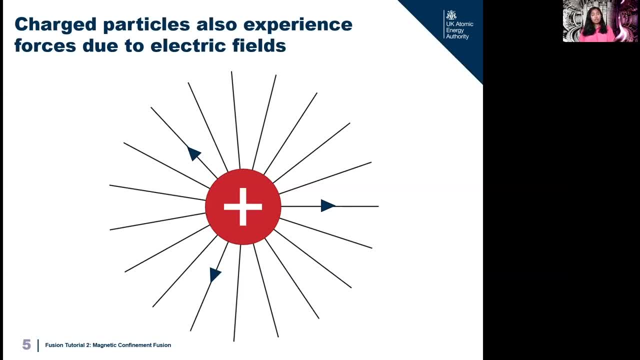 center, the arrows would instead be pointing inwards, towards the negatively charged particle, and this is because we still use the positive test charge particle- here It لو a negative, negative charge- as an indicator of the electric field that the negative particle emits. We can also draw electric field lines for the interaction between two. 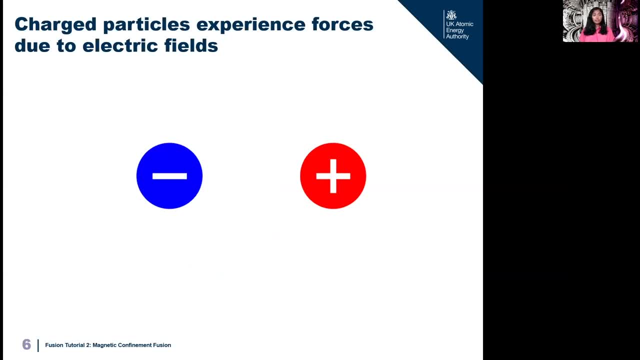 oppositely charged particles, We could have a guess at what the field lines would look like due to these particles using a theory that I've just described earlier. So again, if we place a positive test charged particle here, we know it will be repelled away from the positively charged particle. and if we 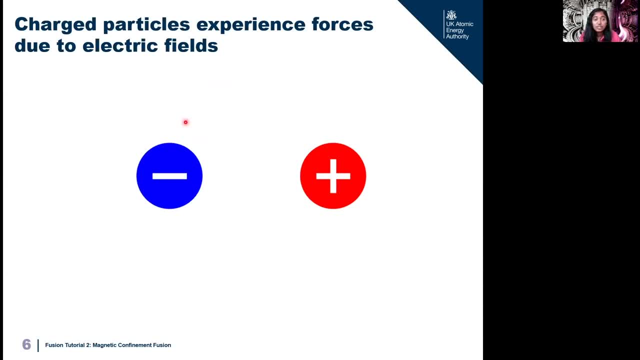 place the positively charged particle here, we know it will be attracted towards the negatively charged particle, like so. So we can imagine arrows going away from the positively charged particle and towards the negatively charged particle and the same underneath, and in general the arrows will be pointing away from. 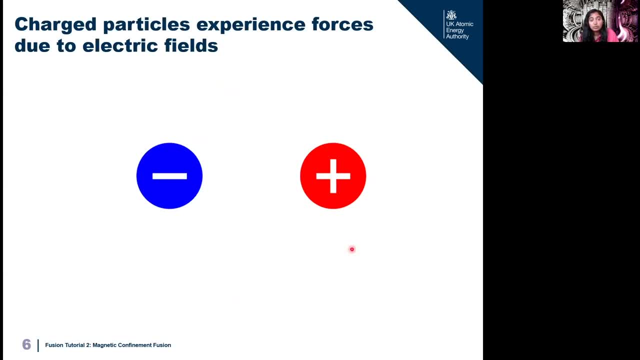 the positively charged particle, because the positively charged particle will be repelled away from this positively charged particle. and here, instead, the arrows will be all pointing inwards, because the positively charged test particle will be attracted to the negative particle. here And here are the arrows behaving exactly as we predicted, So you can see the arrows going all away. 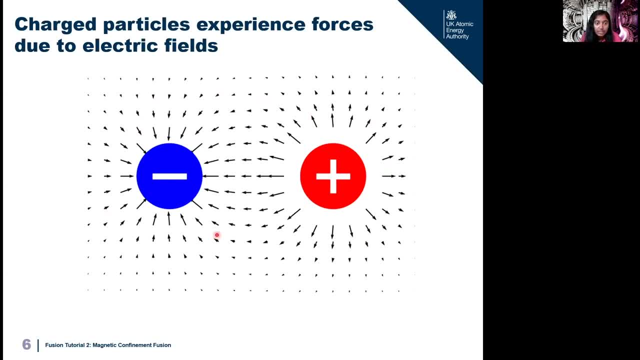 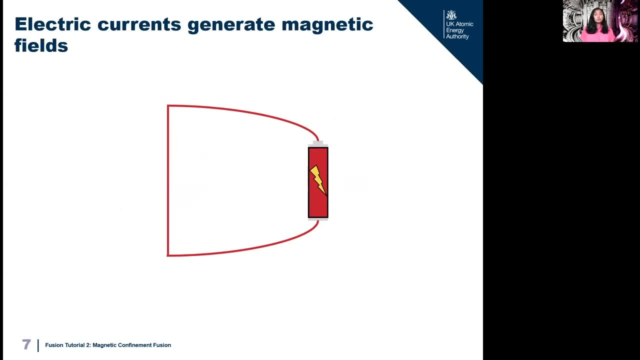 from this positively charged particle and all towards this negatively charged particle here. So how are charged particles, magnetic fields and electric fields all related? Well, if we pass a current through a wire, we can create a magnetic field. So electric currents generate magnetic fields and a current is just charged particles moving around. 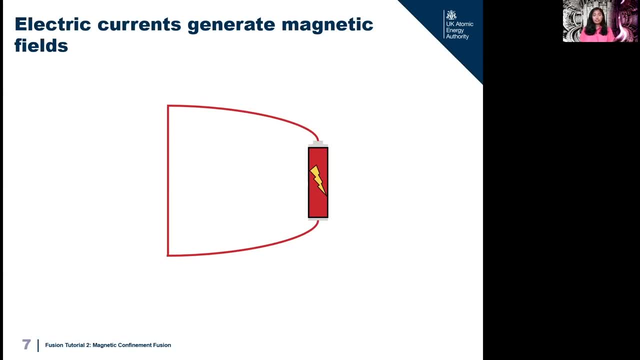 So the straight wire here will create a circular magnetic field. So if we pass a magnetic field- sorry a current- going through this wire, we'll get a circular magnetic field. like so- and this will come in handy later- We can also use this phenomenon to create a straight magnetic field line through the center. So if we 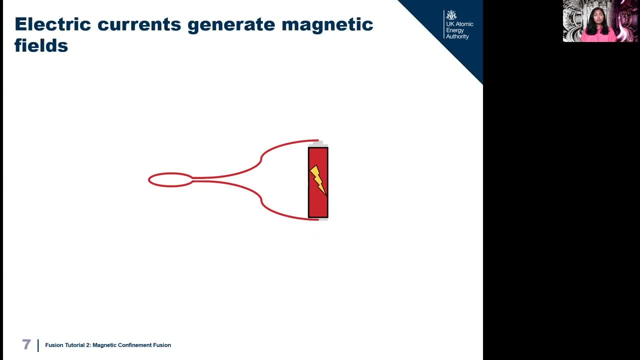 create a loop of wire here instead and pass a current through it, we'll get a magnetic field line. like here And again, this creates a magnetic field line going through the center of the loop itself. Actually, this magnetic field line is the same as a bar magnet would create. 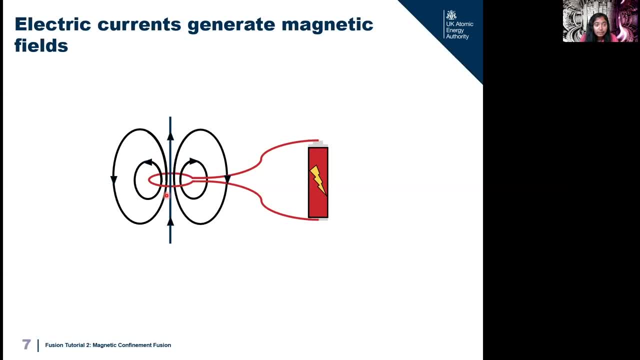 So if here we had the north pole of the bar magnet and down here we have the south pole of the bar magnet, you can see that the magnetic field lines loop around from north to south, like I described earlier. So in this section we've learnt: 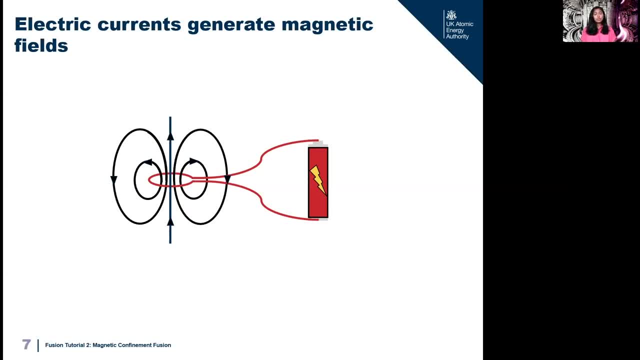 how to draw magnetic field lines due to a bar magnet. We've also learnt how to draw electric field lines due to charged particles, and we've learnt how to draw electric field lines for multiple charged particles. We also found out that electric currents generate magnetic fields and that a current is just the 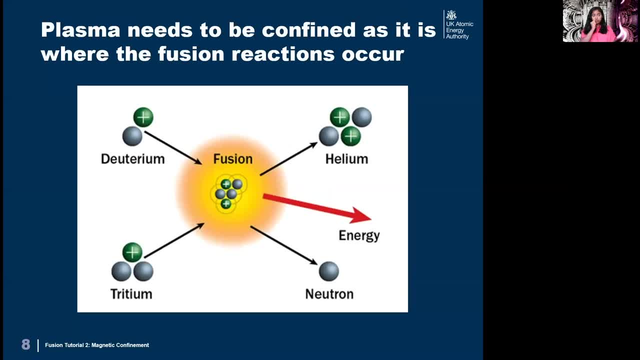 motion of charged particles. So let's bring this back to our plasma. Why does our plasma even need to be confined in the first place? Well, you may remember from the previous fusion tutorial that a plasma is just the conditions we need to create fusion, And 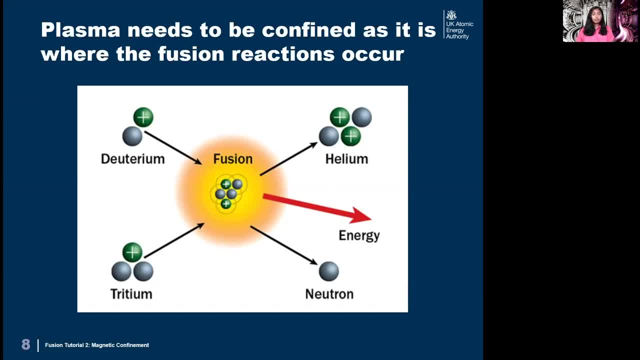 we want to confine our plasma to the current that we need to create fusion And we want to confine our plasma to the current that we need to create fusion And we want to confine our plasma as this is where the fusion reaction occurs. Our fusion reaction is. 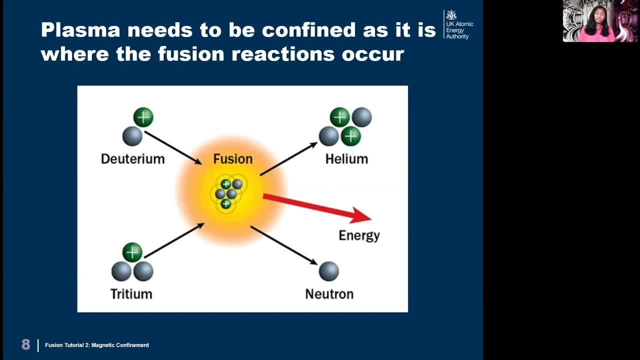 hard to start off and maintain, as mentioned in the previous fusion tutorial as well. so we want to hold it and protect it so that it can burn for as long as possible, so we can get as much energy out of the fusion reaction as possible. We also mentioned in the previous fusion tutorial that our plasma 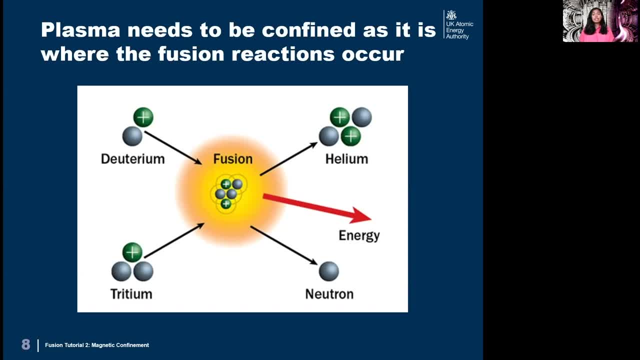 is a gases that is heated up to extremely high temperatures and these temperatures can damage our material and equipment. So we also want to confine our plasma to prevent damage to our material, material and equipment. So we also want to confine our plasma to prevent damage to our material. 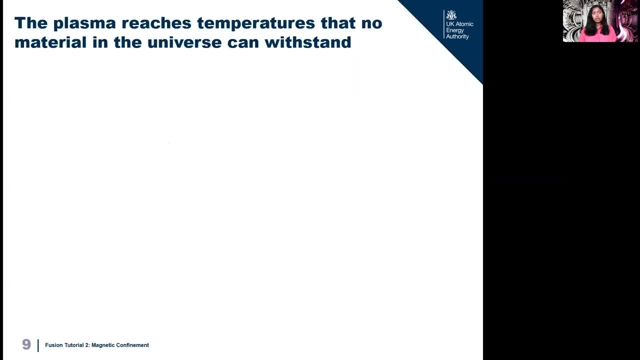 to our material and equipment. As I just mentioned, the plasma reaches temperatures, very, very high temperatures, and actually no material in the universe can withstand these temperatures. So let's compare our fusion machine to the sun, our very own natural fusion machine. We can see that. 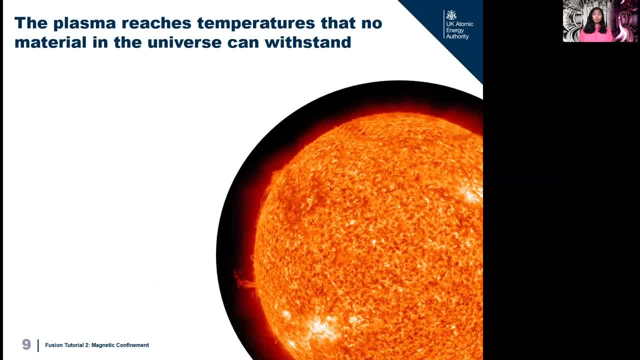 the sun has no container, and this is because it's surrounded by a vacuum, and also because gravity holds it together, keeping the reaction contained. We need to find a way to do this ourselves on Earth, remembering that we're going to reach temperatures much hotter than the center of the 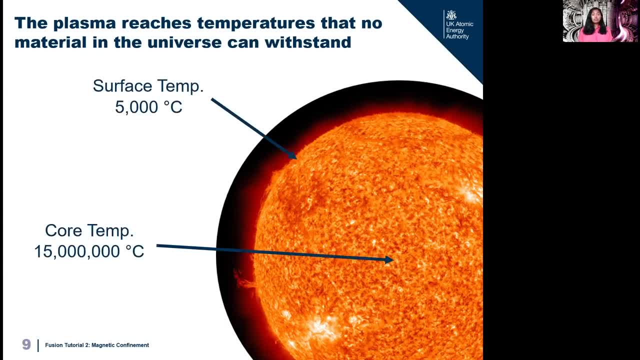 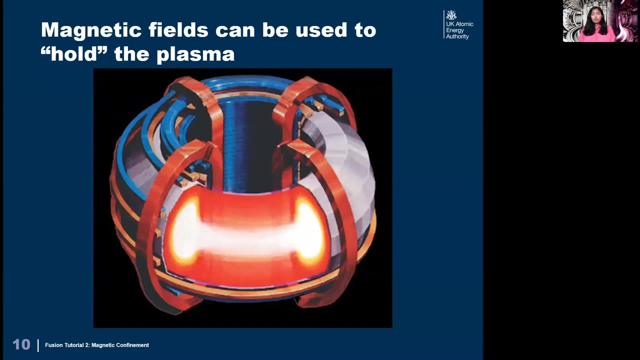 sun which reaches 15 million degrees Celsius, and again, no material in the universe can withstand temperatures that high. This is where magnets come into the picture, as they're a contactless way of holding the plasma, So magnetic fields can be used to hold the plasma. We talked about how 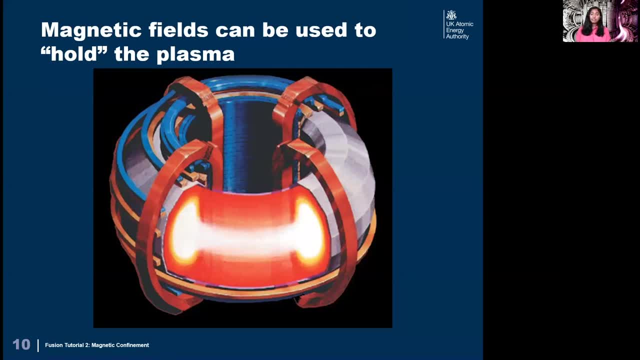 charged particles are affected by magnetic fields, and in the previous tutorial we discussed how a plasma is a gas that's heated up to extremely high temperatures, and how it can be used to trap these charged particles and therefore trap the plasma. The handy part about this is that it 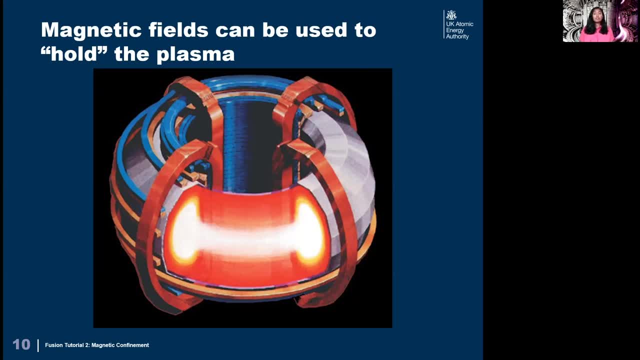 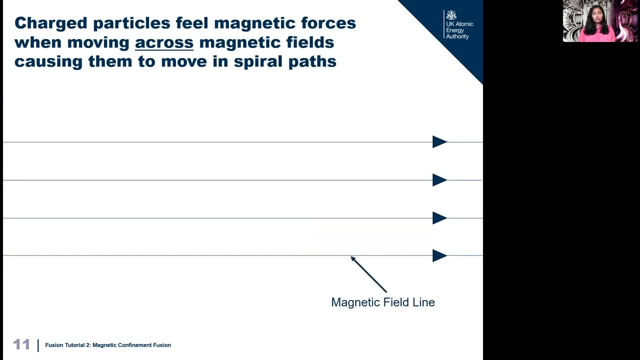 works at high temperatures and enables there to be a contactless way of holding and controlling the shape of the plasma. So how do magnetic fields trap charged particles and therefore hold plasma? Well, if we imagine these lines going across the screen to be magnetic field lines and we place a charged particle in this, 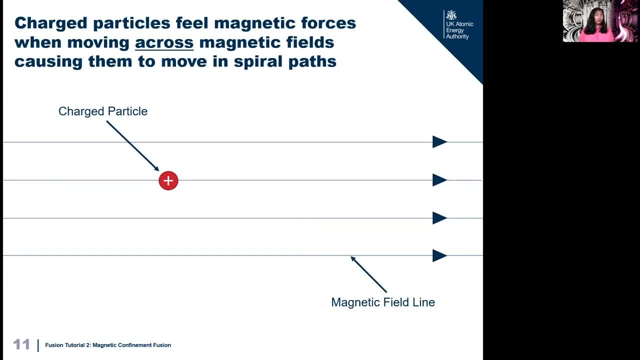 environment. we can see how it behaves and try and figure out how we can use this to our advantage. So if we place a charged particle like so, just still in this magnetic field, it won't have any effect on it due to the magnetic field that it's sitting in, and so it will continue to just sit. 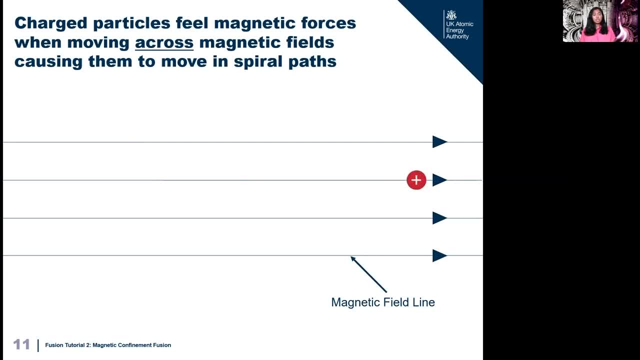 there and remain still. If we nudge the charged particle along a magnetic field line, it will still not feel a force due to the magnetic field and it will continue to move along the line. If, however, the charged particle crosses magnetic field lines like so, then the charged particle will. 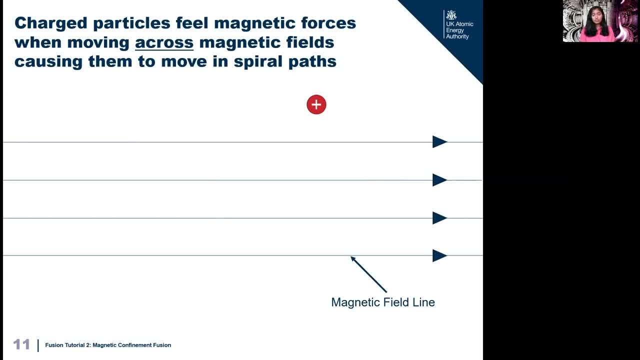 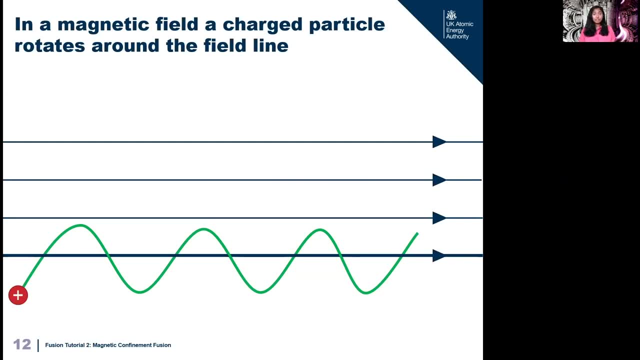 feel a force due to the magnetic field, It will cause the charged particle to move in a spiraling motion like so. So the charged particle crosses a magnetic field line and the force caused by the charged particle crossing the magnetic field line causes the charged particle to 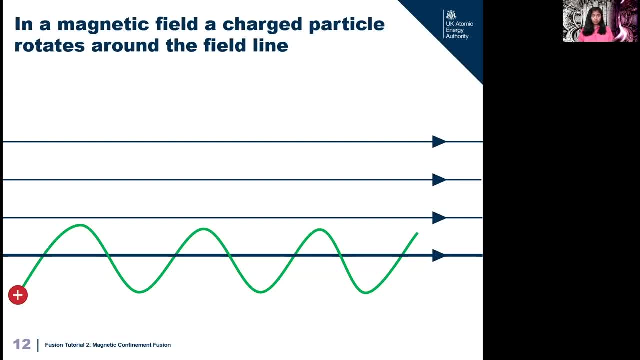 begin moving around the field lines in a corkscrew motion. This effectively traps the charged particle, and the charged particle can only move along the magnetic field line. So to keep the charged particle in this orbit we would have to have an infinitely long magnetic 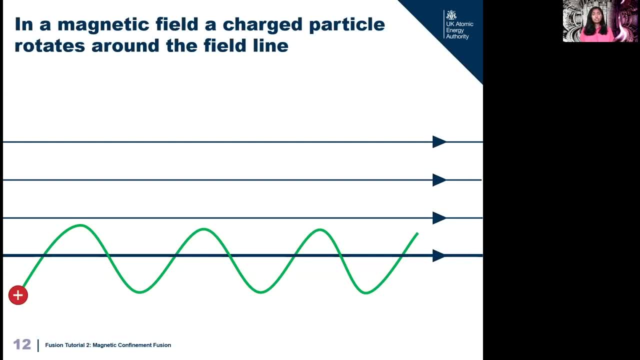 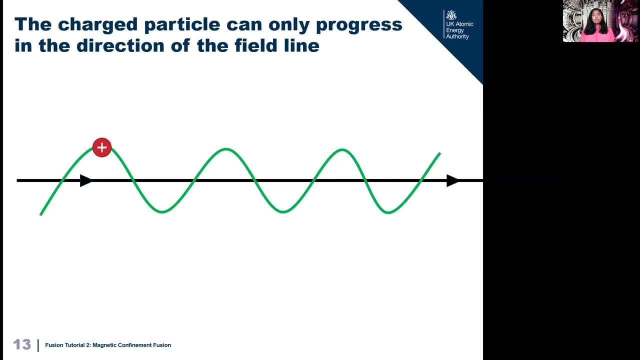 field line, and even a magnetic field line that extends all the way through the center of the earth, wouldn't be enough to contain the plasma for as long as we want to. So, as I just said, the charged particles trapped in an area around this magnetic 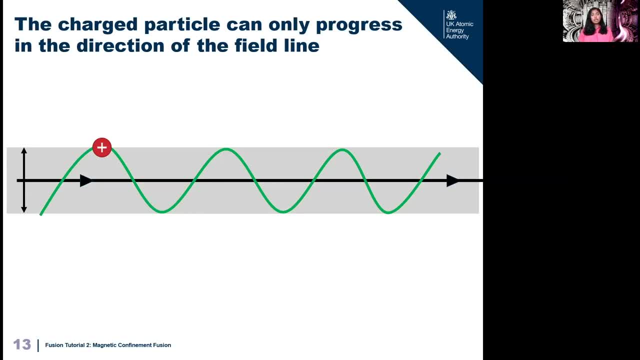 field line, and we can depict this area using this gray box here. However, in 3D, this gray box would be a tube due to the circular motion of the charged particle. So instead of having an infinitely long magnetic field, we could just loop the field line into a circle and keep the 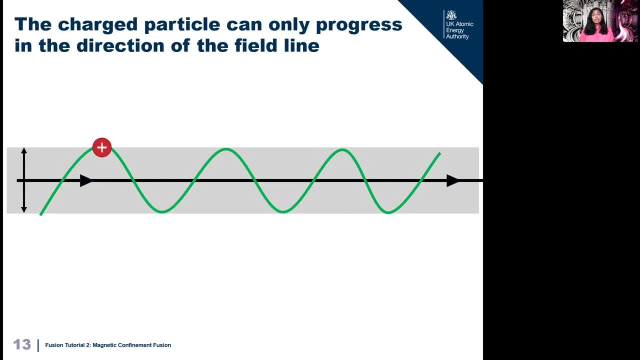 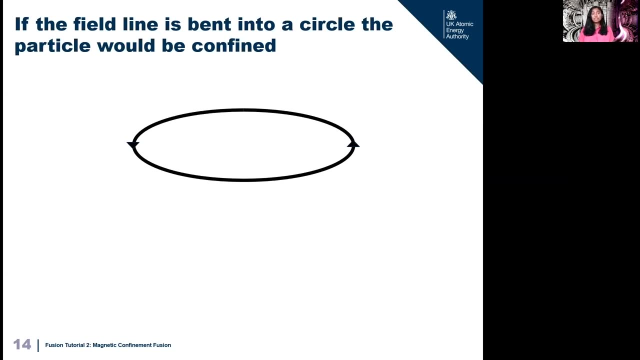 particle trapped in the circular path spiraling along it, and this would keep the plasma trapped for as long as possible so we can get the most energy out of it. So here we have our looped magnetic field line. This is like if we join the two ends of the magnetic field line together And then if we show 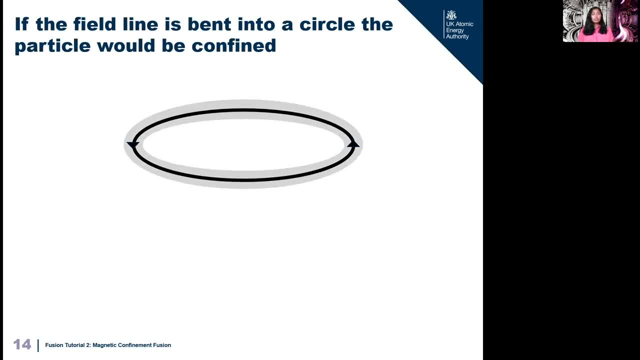 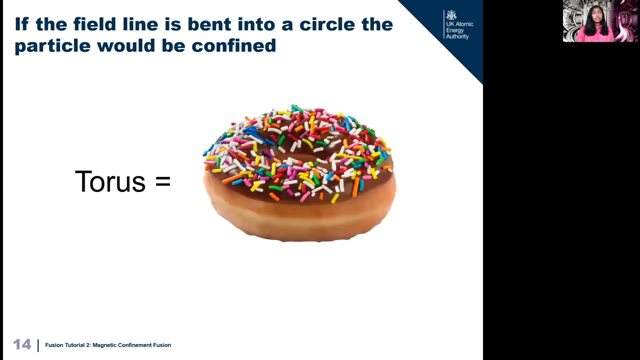 the gray area again of where the charged particles would be trapped. it looks like this And as the charged particles is just what makes up the plasma, this gray area kind of shows the shape of the plasma due to the magnetic field. So this shape looks a bit familiar. It looks like a donut and 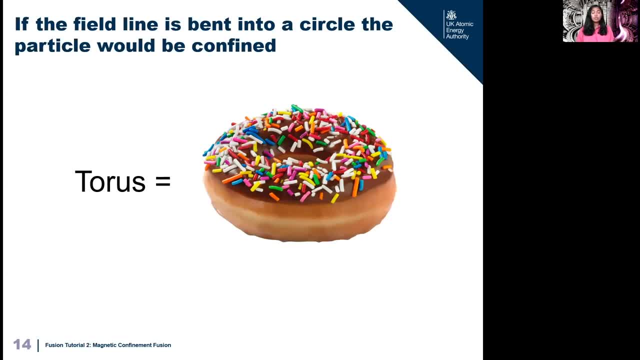 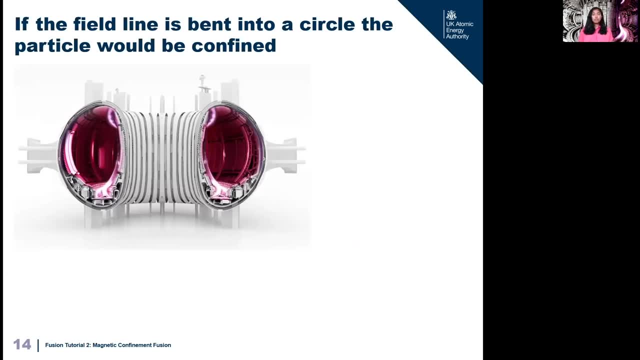 in mathematics, a donut is called a torus. The donut shape is called a torus. This is actually the shape of JET, a fusion machine we have here at Cullinan. You can see this image here and in this image it. 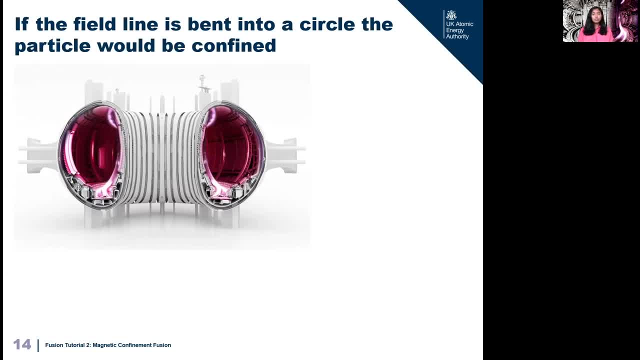 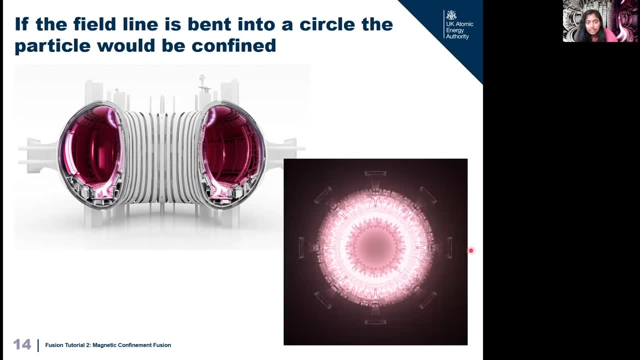 looks like the donut is cut in half, and this is actually our JET at Cullinan. Here's another image of JET from above, and this looks a bit more like a donut, as you can see the ring of plasma here. 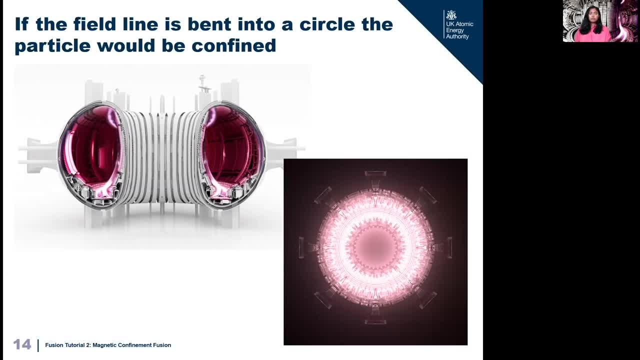 and the hole in the center. So we've made a magnetic field to contain our plasma, but actually it's not perfect yet And this is because the force is strong, stronger in the centre of the doughnut, So around the centre here, the magnetic field. 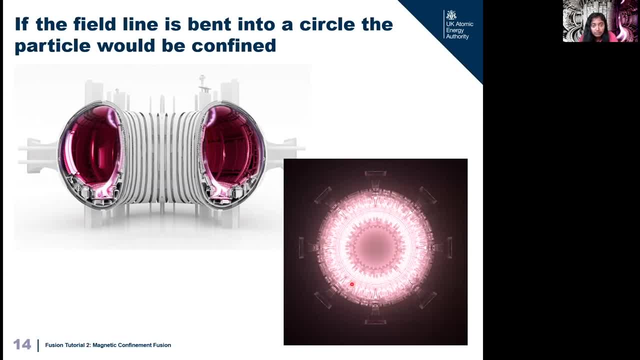 is much, much stronger than it is on the outside of the doughnut. here This means that the particles are being thrown towards the outside of the doughnut, So we have a plasma that leaks out of the edges of the doughnut. If you imagine a bucket being 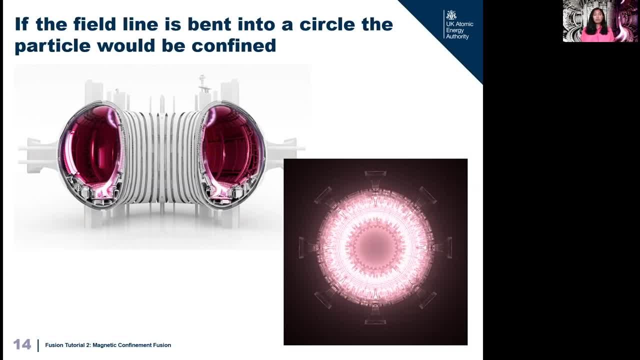 spun above your head. the water in the bucket is being thrown to the bottom of the bucket and held in place by the bottom of the bucket, And this is what stops you from being soaked by the water. Similarly, the plasma is spinning round and round in this doughnut shaped container. 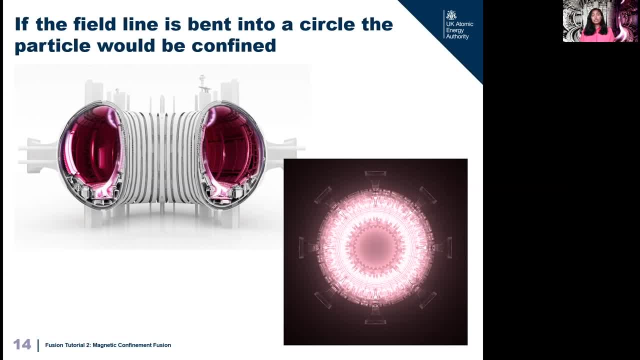 but the plasma is being thrown towards the outside of the doughnut And we need to figure out a way to stop it from leaking out, in a way like using the bottom of the bucket to stop it from leaking. So, to stop the plasma being thrown out, the 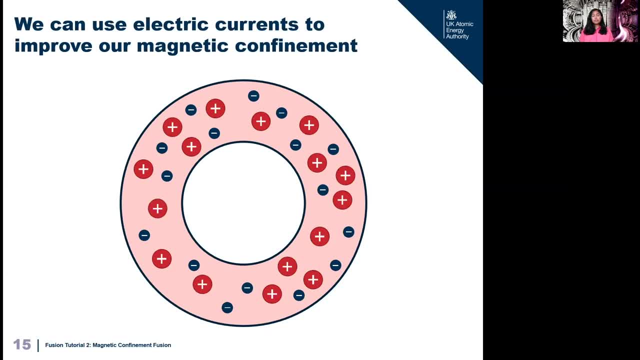 edge of the doughnut, we can induce a current in our plasma And this electric current improves our magnetism. We can do this by using a big transformer coil down the centre of the doughnut. If you watch the next fusion tutorial, you can find out a bit more about transformers and how. 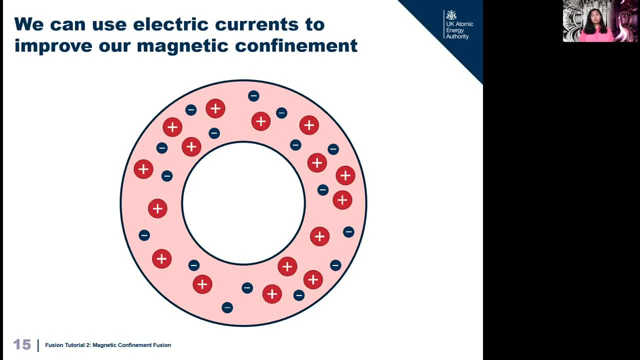 they work and how inducing a current in the plasma heats up the plasma itself, If we remember from previously that an electric current is just the movement of charged particles and we know that our plasma is made up of charged particles. So here our plasma is. 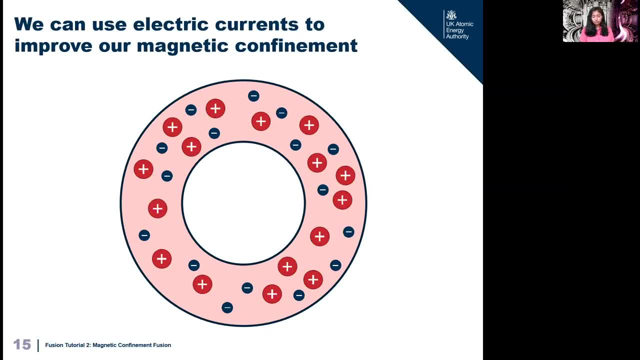 behaving like a loop of wire, like we saw earlier. So if we induce a current in the plasma, it will heat up the plasma itself, And if we induce a current, the charged particles start moving like so and our plasma is basically the wire. 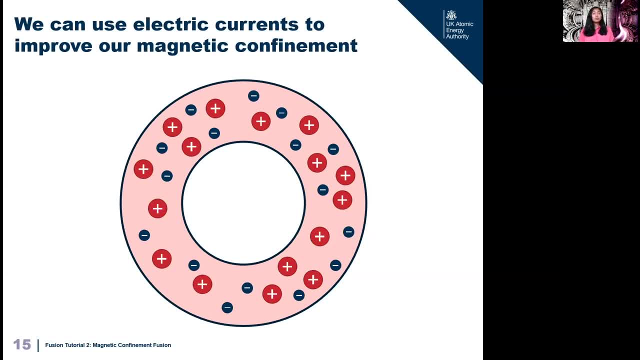 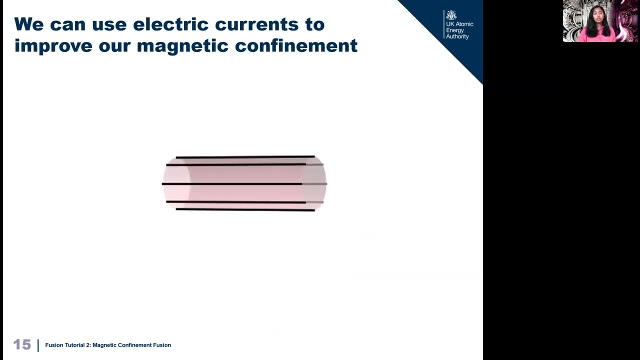 So this current creates a magnetic field that loops through the centre of the doughnut. So if we uncurl the doughnut like so, the magnetic field lines would look like the red lines here looping through the centre of the doughnut. So in addition to the magnetic field lines we looked at that go around the doughnut, the 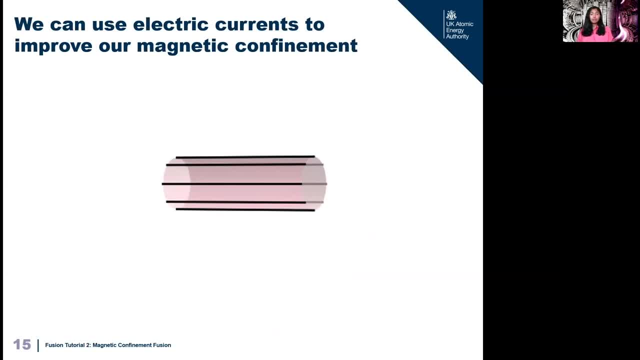 long way. that look like this: you have a magnetic field that loops around the short way through the centre of the doughnut And these combined together create a twisty magnetic field like so, And this holds the plasma a lot better and keeps the plasma a lot more stable. 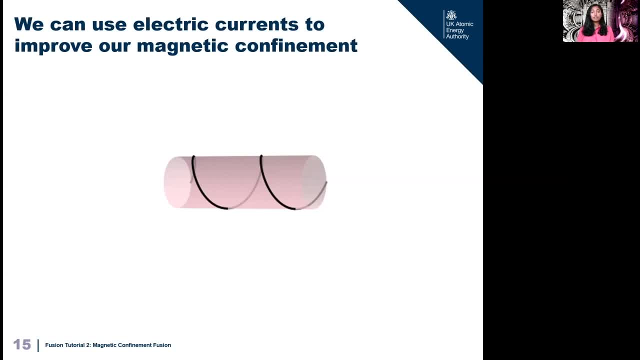 It also means that we can stop the plasma being flung towards the outside of the doughnut and therefore reduce the leakiness of the doughnut-shaped plasma, And therefore we can have a plasma that burns for longer and get more energy out of it. 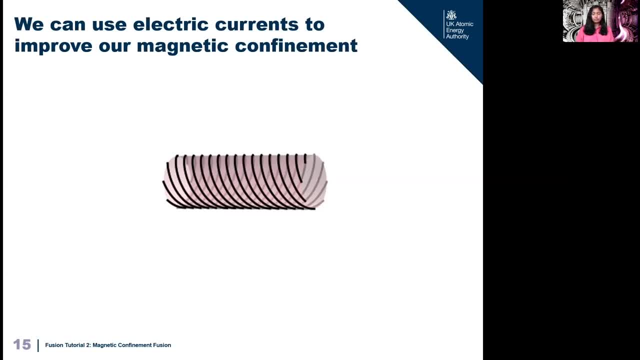 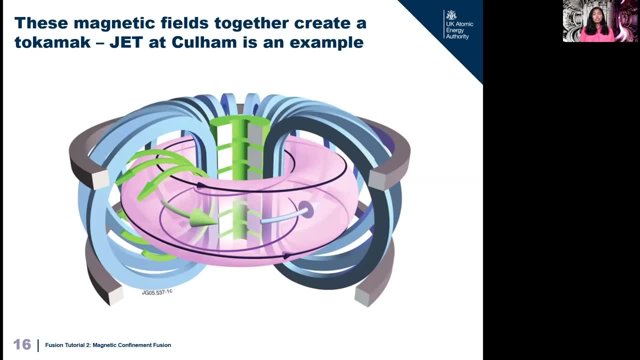 If we draw all the field lines around the doughnut, it would look a bit like this. If we draw all the field lines around the doughnut, it would look a bit like this: So these magnetic fields combine together to make a plasma that looks like what we have. 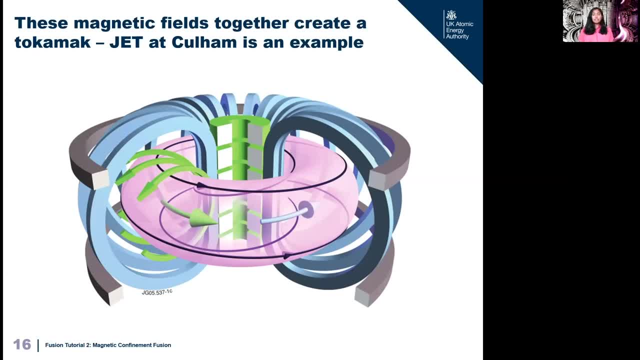 here at JET in Cullin. This style of fusion using these magnetic confinement methods is called a tokamak, and this is a Russian acronym, which basically means a torus-shaped fusion reactor or a doughnut-shaped fusion reactor. You can see that these blue D-shaped coils create a magnetic field that goes around the 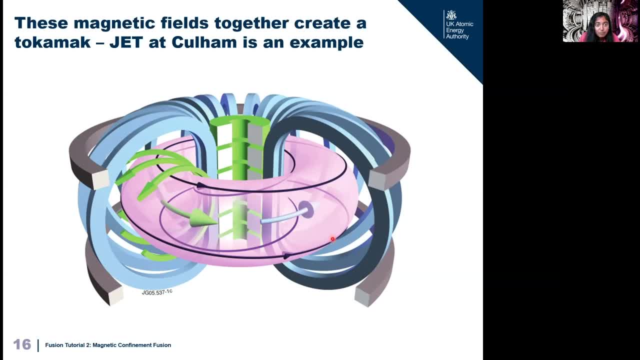 centre around the long way. So this is a T-shaped fusion reactor And this plasma in pink here is. then. then we have a transformer coil in the centre that induces a current in the plasma itself, shown by this green arrow here. This current in the plasma then induces the magnetic field lines that loop through the 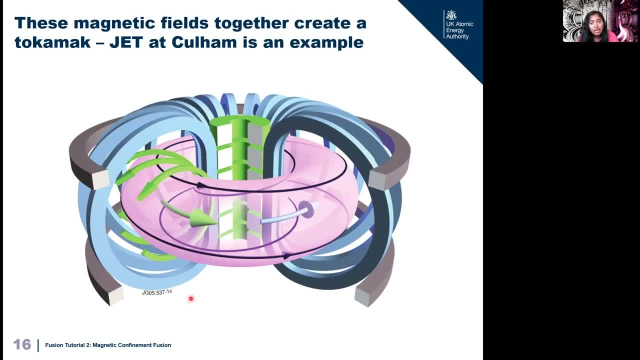 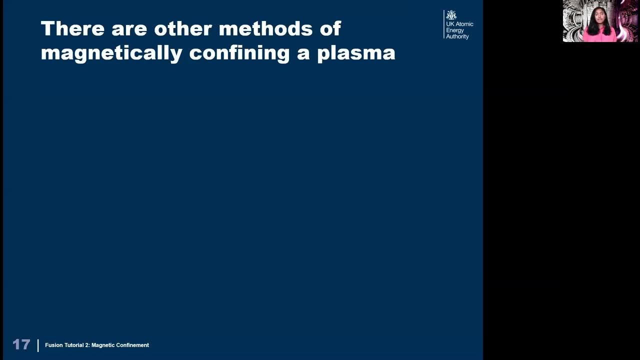 centre of the doughnut, as I mentioned here, shown by these green arrows here, And in total this creates a plasma that's a bit more stable than if we didn't have the plasma current in the centre. So now that we've learnt one method of magnetically confining a plasma called a tokamak, are 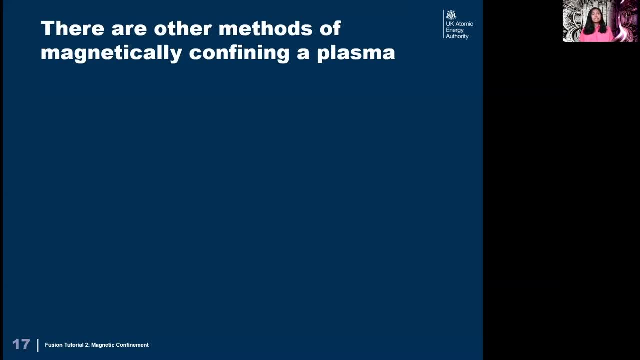 there any other methods of magnetically confining a plasma? Yes, actually there are. We even have an example right here at Cullin and it's called MAST-U. This type of magnetic confinement technique is called a spherical tokamak. 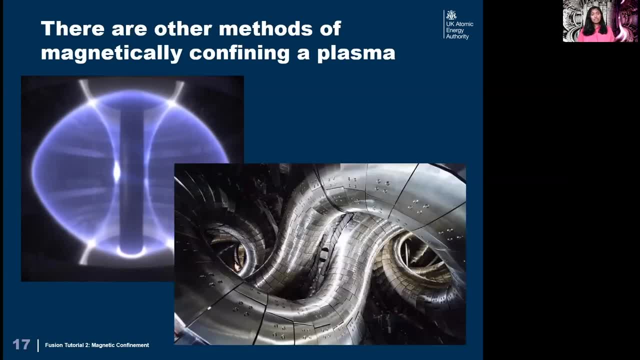 There are also other examples around the world, for example, a stellarator, this funky-looking fusion machine. Let's have a little look at these techniques And how they differ from the ones that we use at JET, the tokamak. 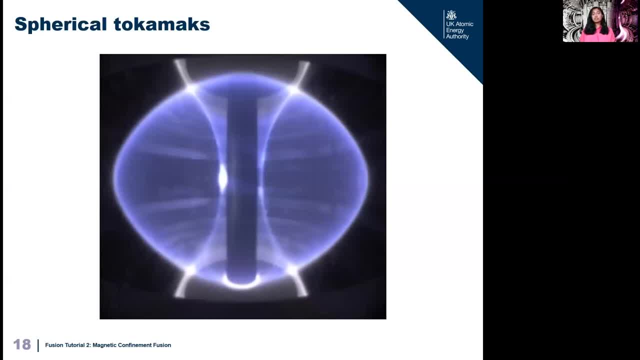 Let's look at spherical tokamaks first. The spherical tokamak is based off of the tokamak principle that we used for JET. It basically takes the tokamak's doughnut shape and tries to reduce the size of the central hole as much as possible. 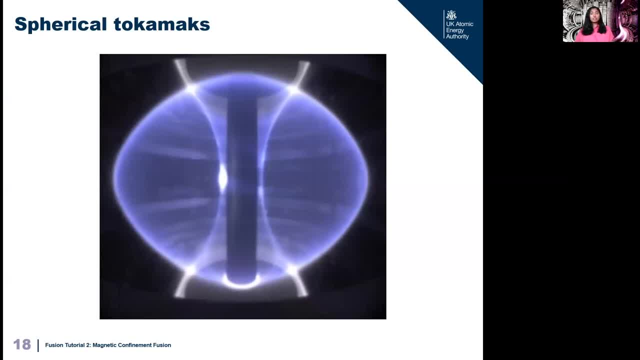 It does this by having the magnets as close as possible to the plasma, whereas in tokamaks the magnets are a little bit further away from the plasma. This results in a plasma that is a bit more spherical in shape, as you can see here. 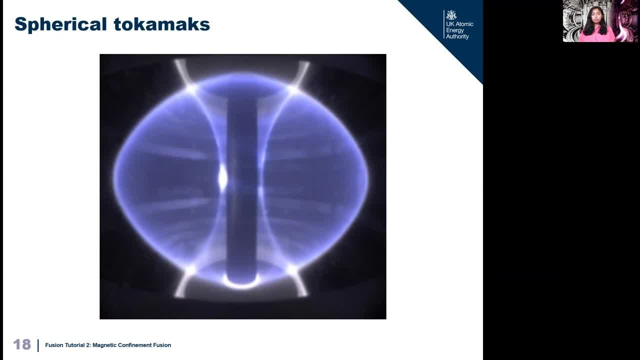 It also has a more spherical shape. as you can see here, It also looks a bit like a cored apple. The principles of the spherical tokamak in terms of magnetic fields are the same as a tokamak, But because the plasma is much smaller, you need less magnetic field in comparison to 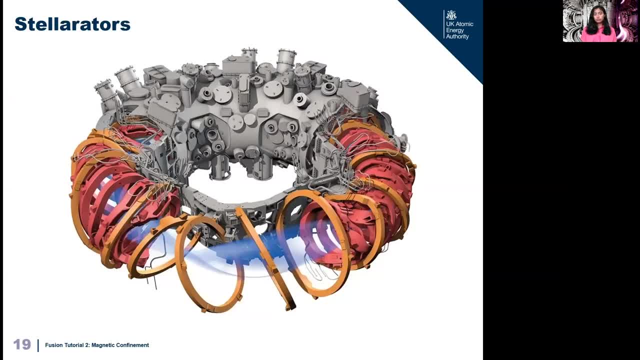 JET to produce a stable plasma. Let's talk about stellarators next. Stellarators are actually one of the earliest ideas for a way to magnetically confine a plasma. They were originally scrapped as they were too difficult to design, but after the leaky 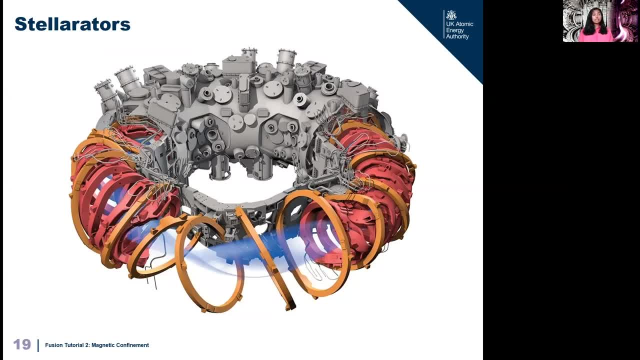 plasma issues and the development of computers and supercomputers, the interest in them took off again. The twisting shape of the plasma, as you can see here in blue, eliminates some of the leaky plasma issues that the doughnut-shaped plasma had that I mentioned previously. 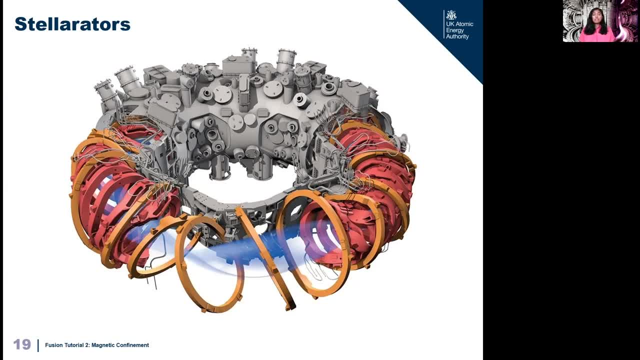 Because this plasma is a lot more stable. the plasma doesn't require a current going through it, as the twisty shape of the plasma makes it a lot more stable. Therefore, you don't need a transformer in this case. The plasma is a lot more stable and the plasma doesn't require a current going through it. 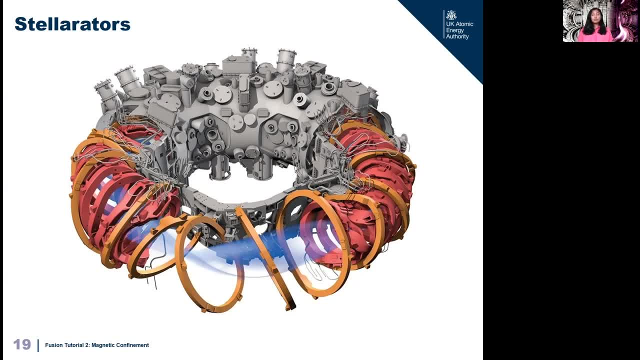 Therefore, you don't need a transformer in this case. The plasma is a lot more stable and the plasma doesn't require a current going through it. In theory, this is the case for the plasma in the center of the stellarator and, as 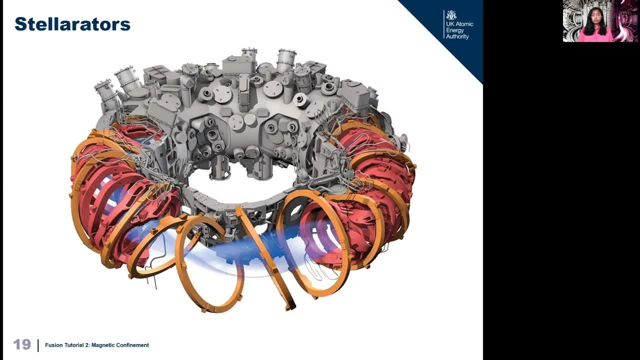 transformers require a lot of electricity. they make stellarators a lot cheaper to run. In theory, the plasma could last for ages, but they are a lot more difficult than a tokamak. Stellarators are often said to be a physicist's dream, but an engineer's nightmare. 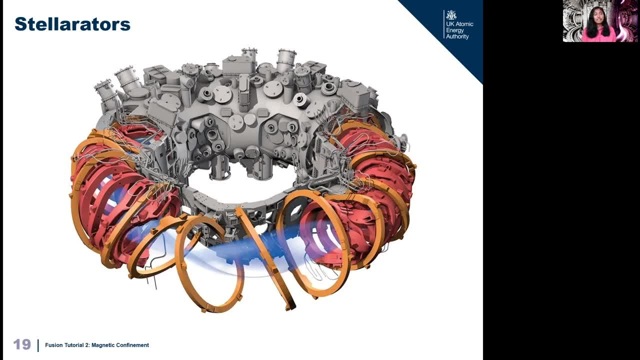 This is because the stability of the plasma makes a stellarator a physicist's dream, but the complexity of building a stellarator in real life is an engineer's nightmare. At least for me, it's the same.